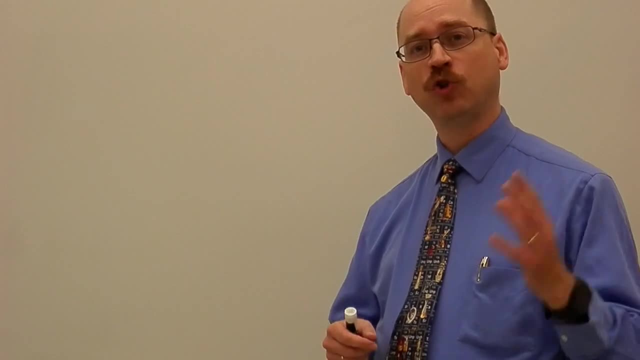 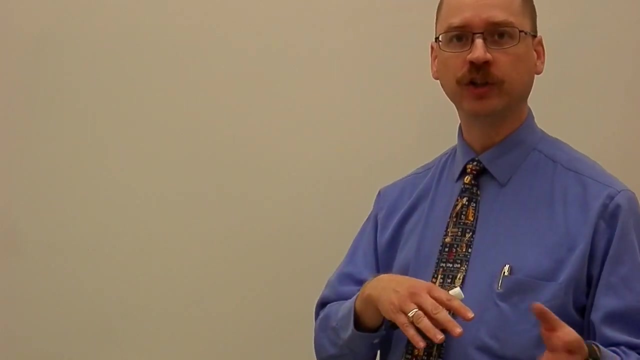 you will get to the right answer. The other thing to keep in mind is try to do bed mask backwards. So start with the addition, subtraction, Then work into doing multiplication, division. Leave any brackets or exponents until pretty much last, if you can. 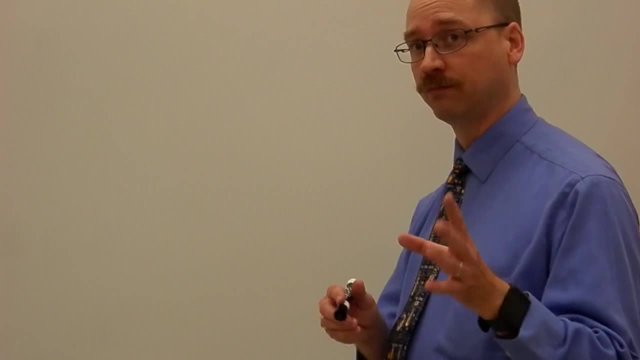 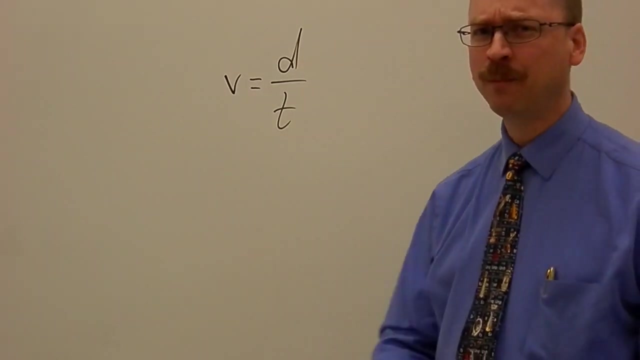 I'm going to show you the most famous formula in all of physics just to get you started, And that's the formula: V equals D over T. Now, sometimes people will tell me about putting this in the triangle, and then they solve it. 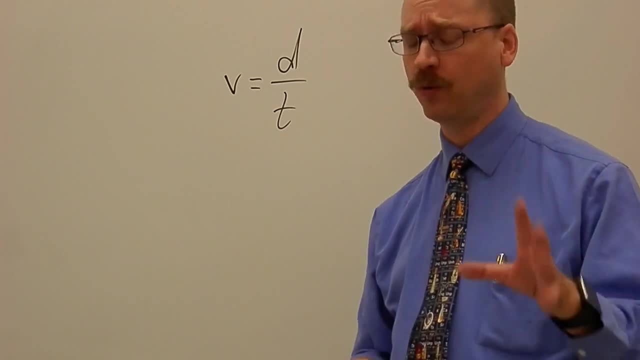 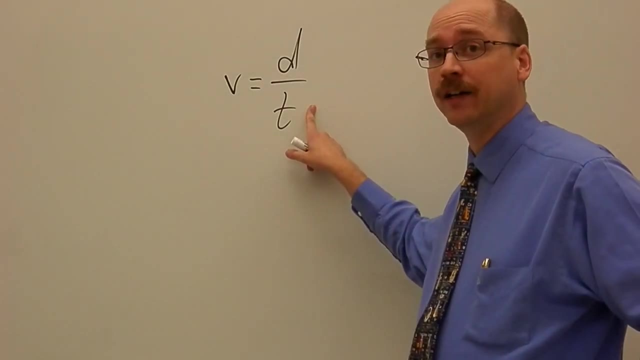 If you don't know what I'm talking about, don't worry about it, because that's good. I don't want you using the triangle, But using this formula with the triangle thing isn't a great idea if you have been using it. 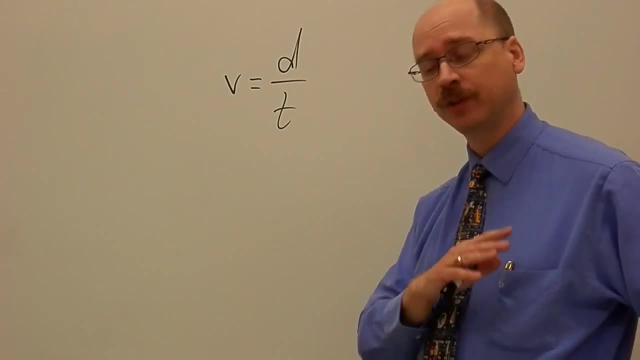 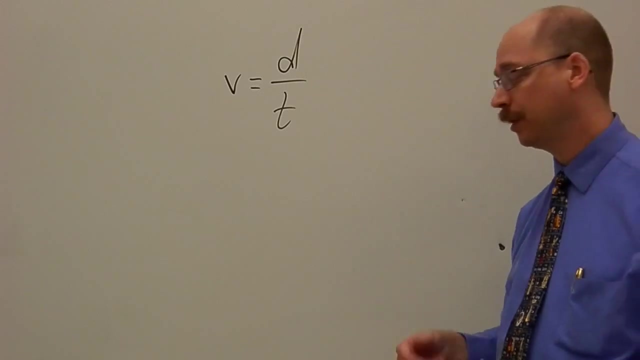 because most of the formulas don't work that way. So let's not even try it, Let's not even get into it. Instead, I tell you that in this formula, I want you to solve it for D, the displacement. So what I'm looking at is I want to get D all on its own. 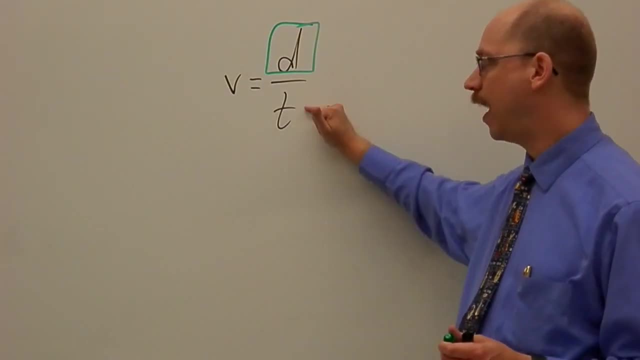 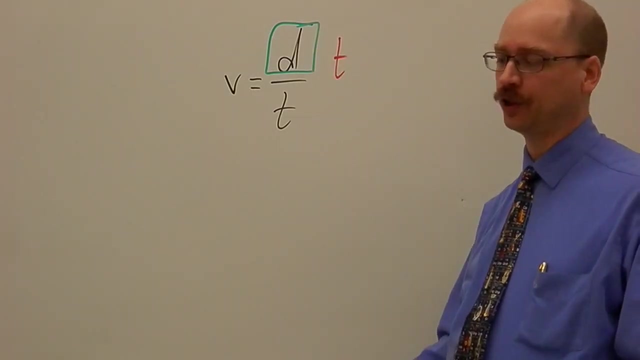 What's the one thing being done to D right now? We're dividing it by T, That's it. So I'm going to multiply by T, because that's the opposite of division. I'm going to do the same thing to the other side. 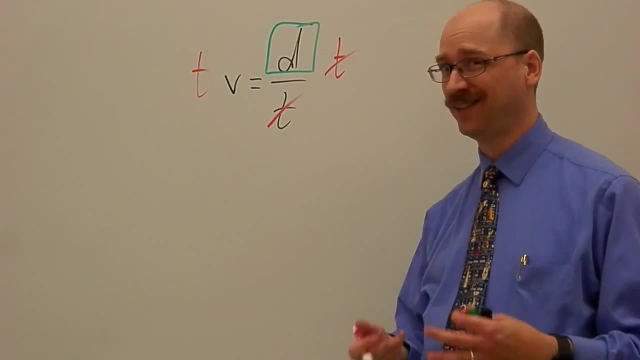 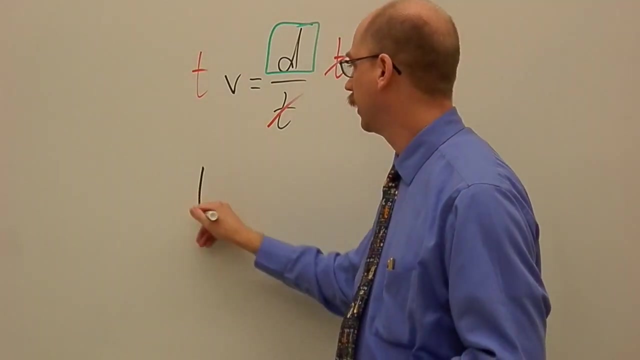 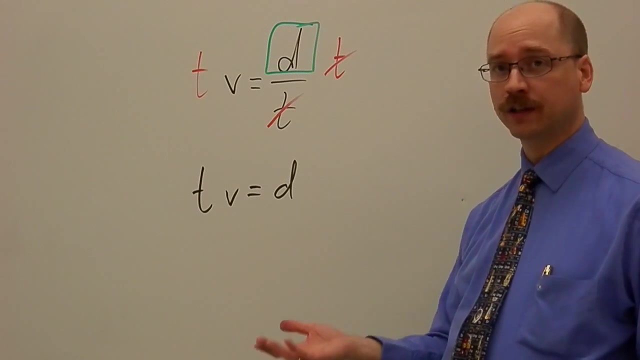 T and T. D divided by T equals 1.. It cancels. I don't get rid of it on this side because it's not cancelling on the other side. This would leave me with the formula: Tv equals D As a general rule, and this is just sort of the way that we do things in physics. 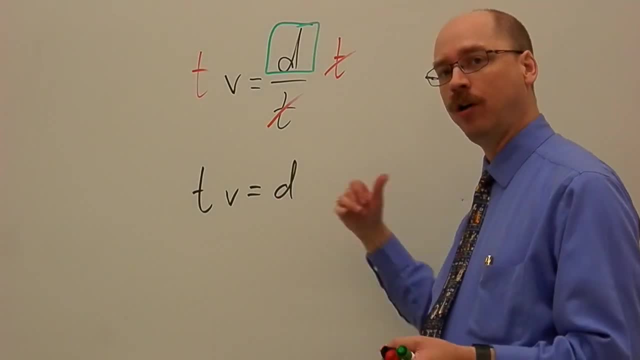 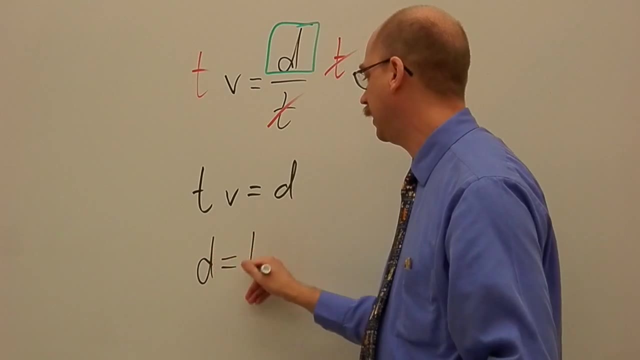 similar to math. we don't leave our unknown variable on the right-hand side, So that means that usually what I'll do is I'll just flip this whole thing around And I'll write it as D equals Tv, like that. 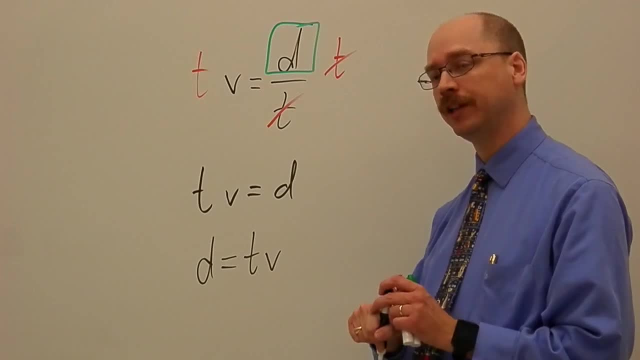 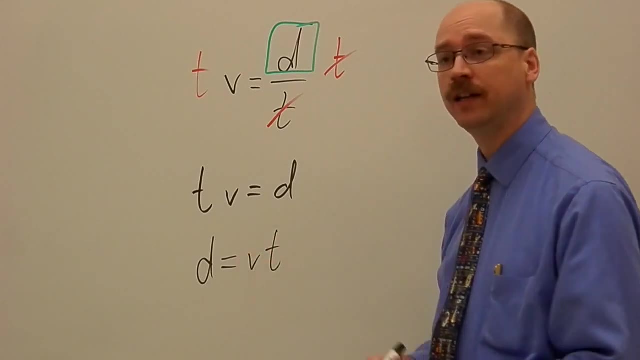 So displacement equals time multiplied by velocity. If you want to, or if this is just the way that you wrote it out, if instead you've got Vt, it's the same thing, Because when we're multiplying these two variables on the right-hand side, 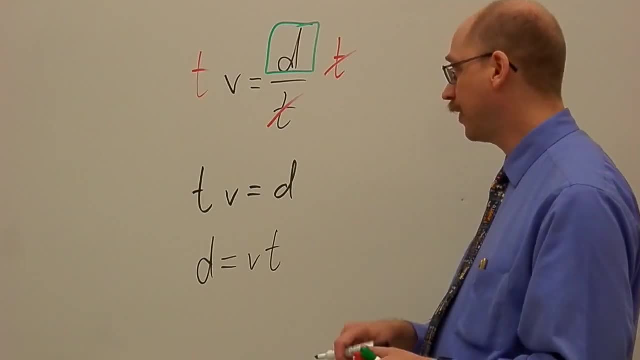 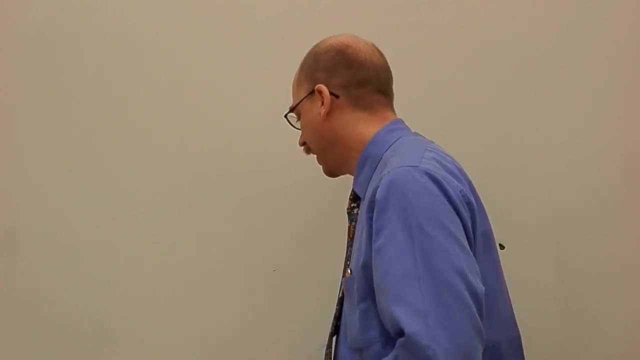 it doesn't matter what order we're multiplying them in. So we've got that formula. Now if I was instead trying to solve it for T? I usually get people doing a little bit of a mix-up here, because what they don't remember is T is in the denominator. 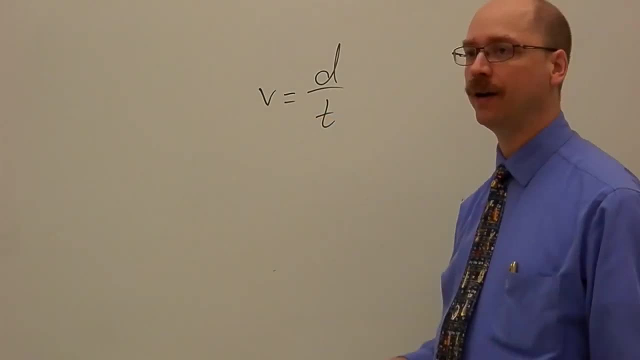 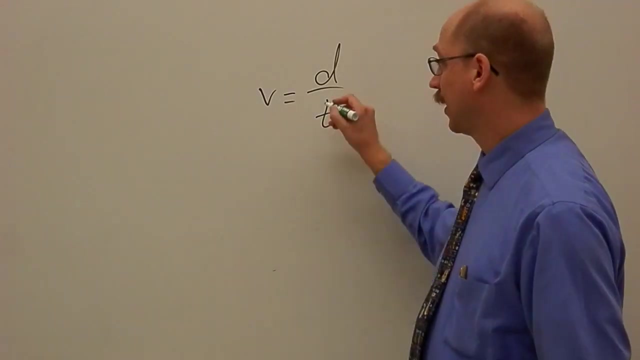 So that means that I can't just say, oh, I'll divide by D, divide by D- T would still be on the bottom. We've got to move T up first. So this will sound a bit kind of redundant because we just did it. 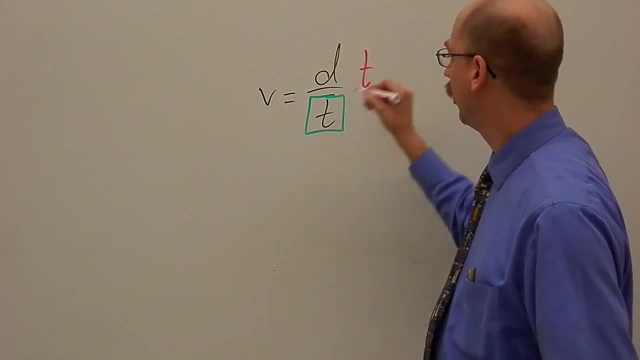 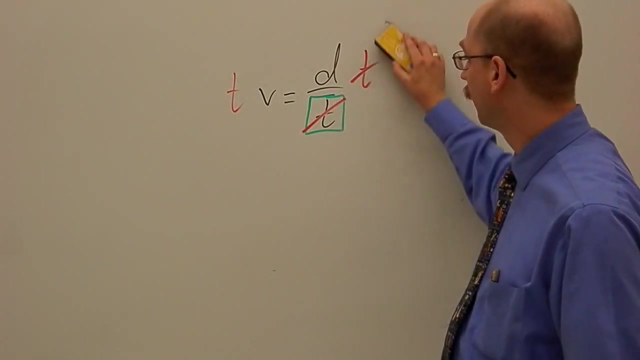 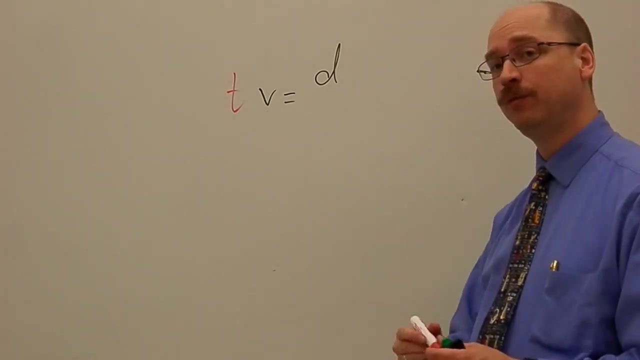 but if I'm solving for T, I'll multiply both sides by T again, These Ts cancel, and remember that happened before. So I get something that looks like that. Now what I need to do is still get the V to move over. 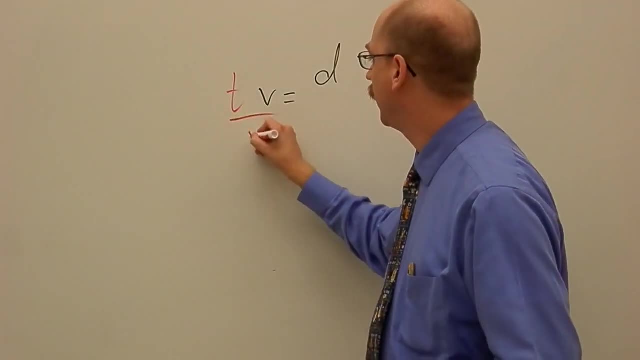 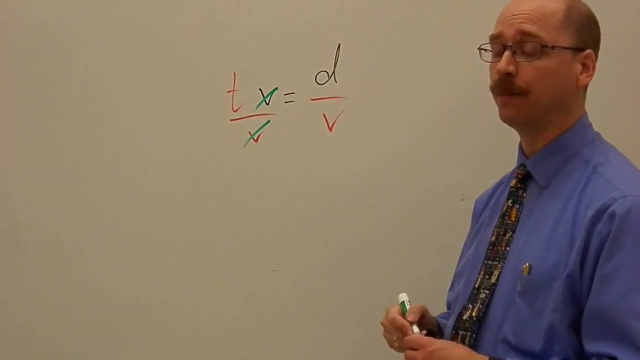 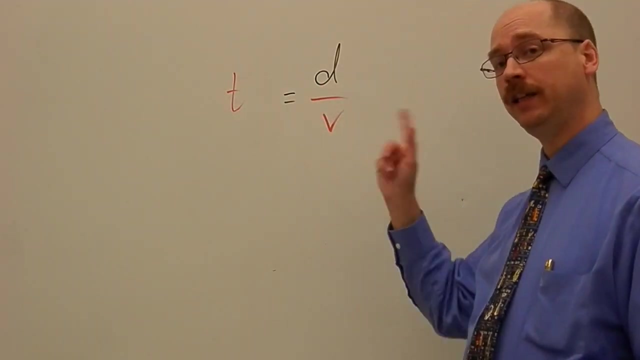 because I'm trying to isolate T on its own. Divide by V, divide by V. These Vs, divide by V, equals 1. They cancel, and now I've got the formula I need: T equals D over V. Good to go. 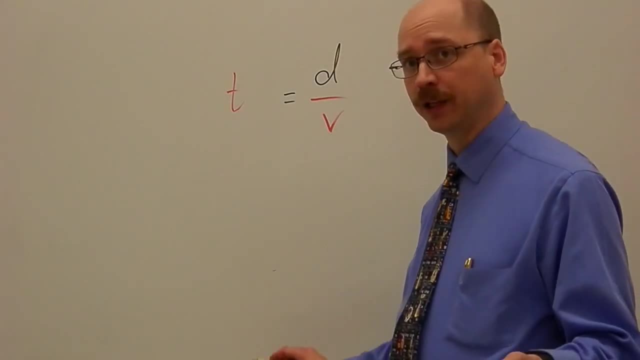 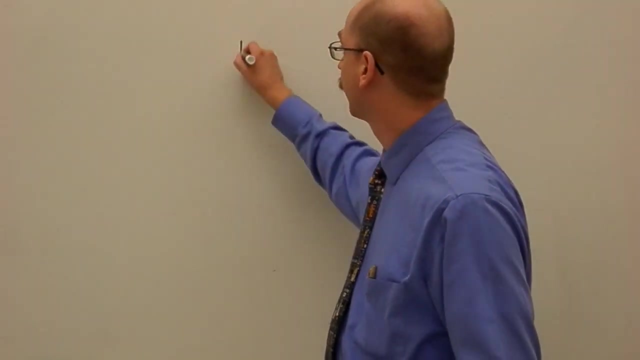 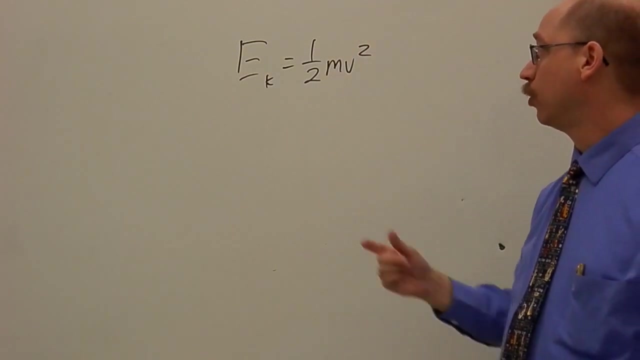 Now, that is the most basic formula out there that you should have to do some manipulations with. There's another one that I'm hoping you remember from science: 10. Ek equals 1 half mv squared. If I'm solving this one for, let's say, for example, m. 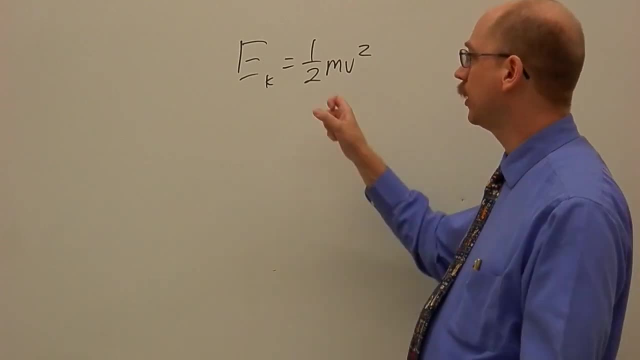 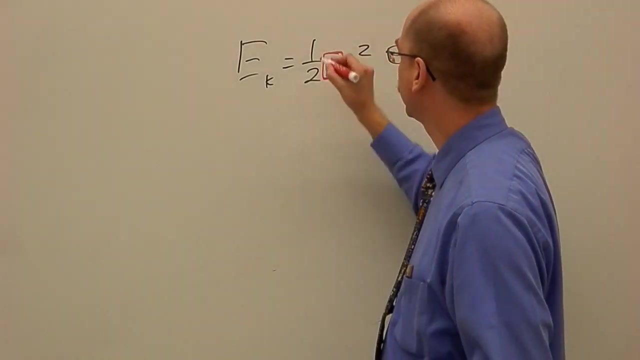 I've got a couple of things I've got to move around Myself. usually I go after this 1 half part first. I just don't like seeing that there. So if I'm trying to isolate for m, the first thing I'll do on its own to get just this silly fraction out of the way. 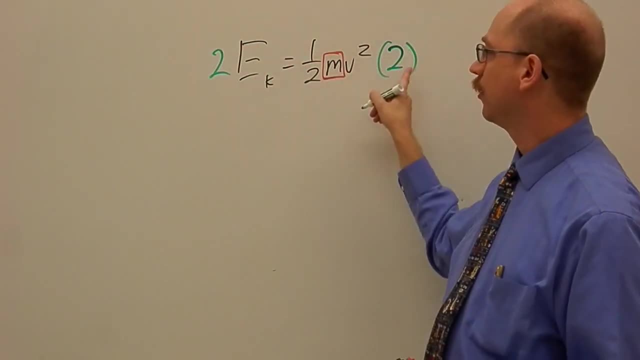 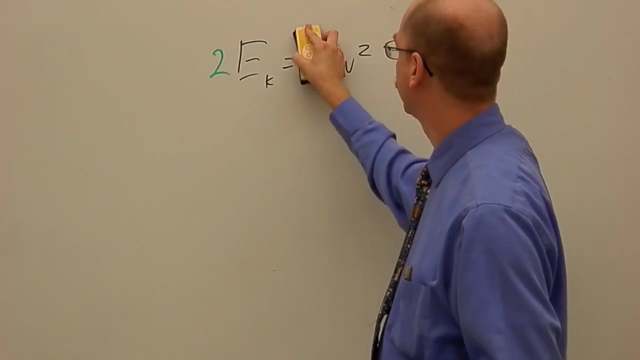 multiply both sides by 2.. Now I threw this all the way over there, but really it's 2 divided by 2. So that cancels and it leaves me with that. I still need to get the V squared to move. 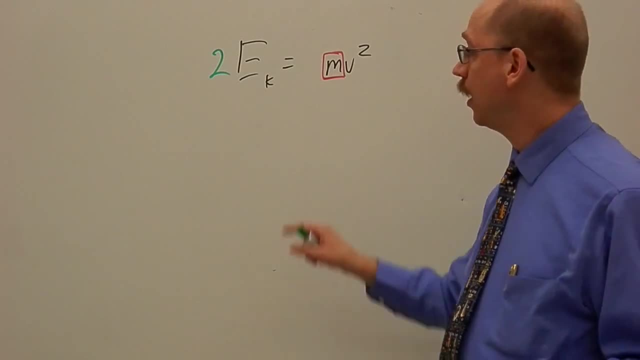 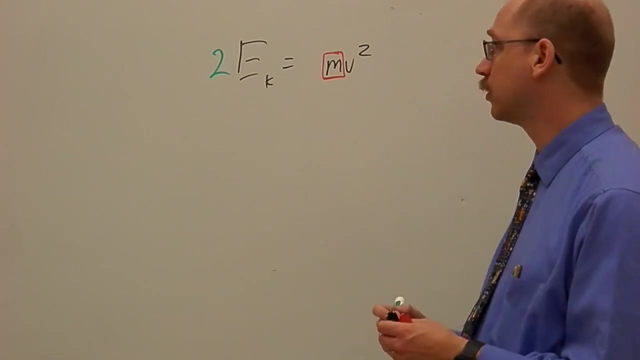 and sometimes people worry about this. They say, well, I just square root it now. No, If I'm solving for m, I get to leave V alone. So all I have to do is just move it to the other side as one big clump. 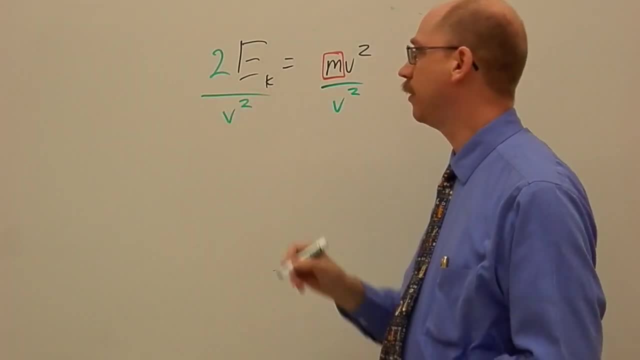 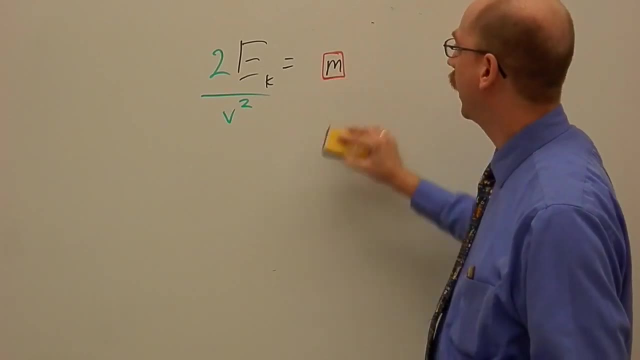 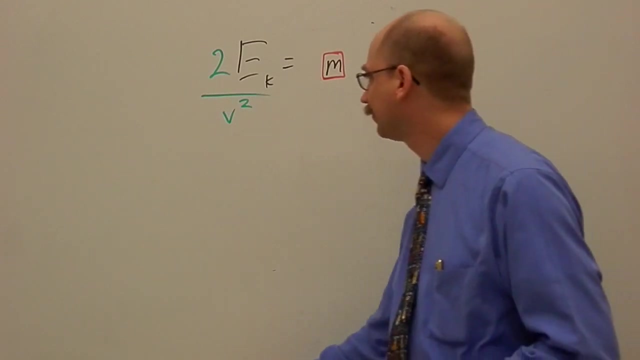 So divide by V squared, divide by V squared Over here. V squared divided by V squared cancels and leaves me with m. 2 ek divided by V squared equals m. I'm set. What if, though, we had to solve that same formula for v? 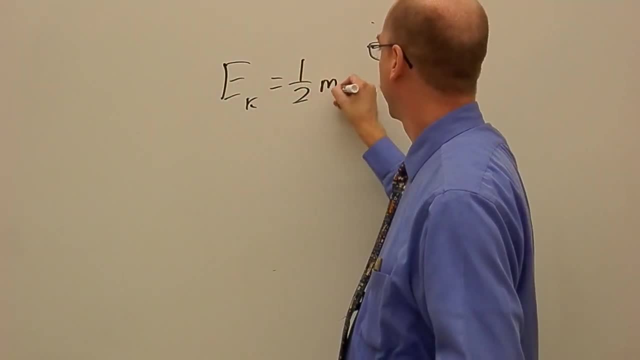 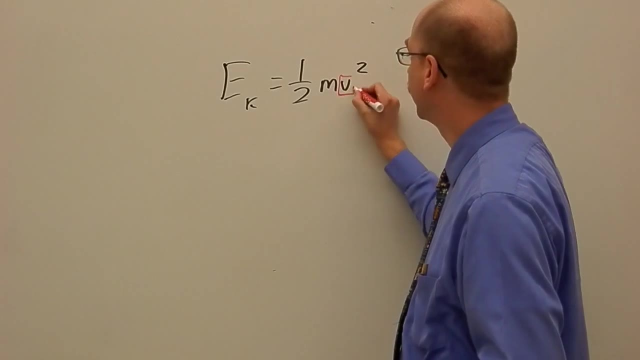 If we're doing that, then we do have to be a little bit worried about that V squared. I still get to do the same thing as I'm trying to isolate just V on its own. I still get to do the same thing with the 1 half. 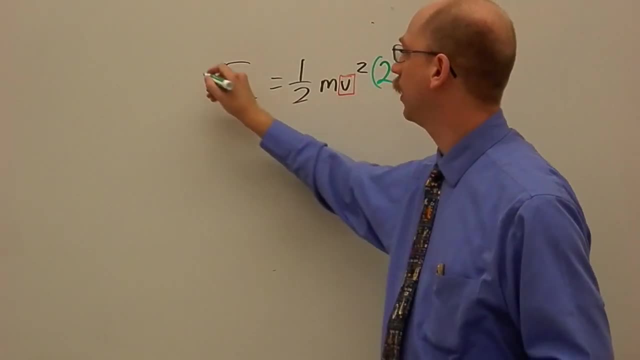 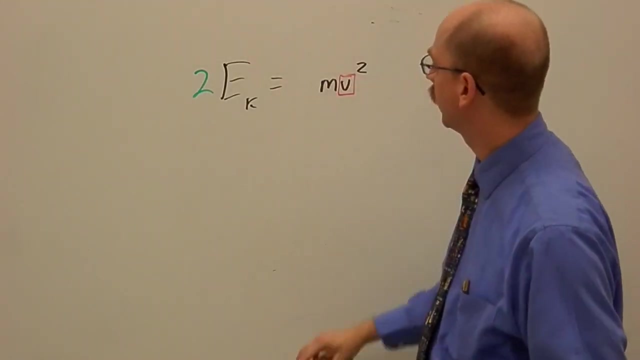 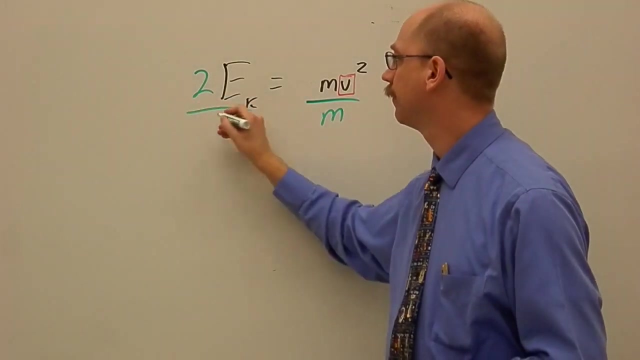 I still need to move that. So multiply by 2,, multiply by 2.. 1 half and 2: cancel. Now I'm going to have to get rid of that. m get that moved to the other side. Divide by m. divide by m- m over m. 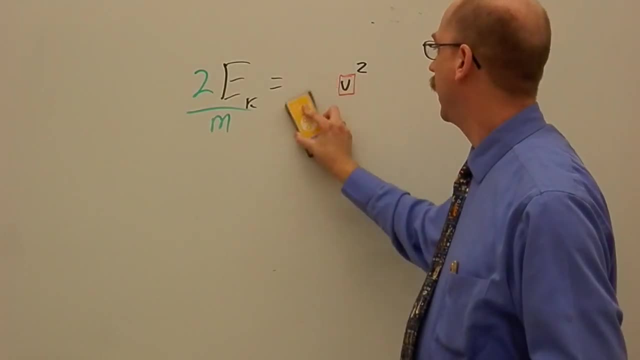 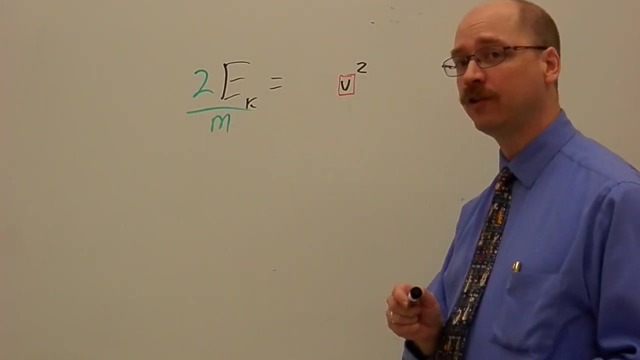 Equals 1, so it cancels out. And now the very last stage in this. I can't have V squared, I need just V Now, mathematically, this is a bit of a dangerous thing to do. Your math teacher will tell you. 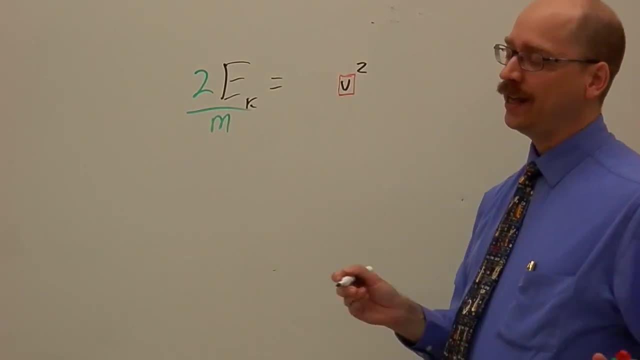 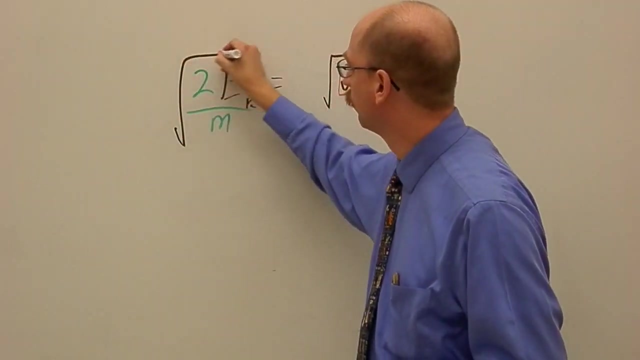 watch out, because you don't know if that's positive or negative V value In physics. we're going to rig it, so that's not an issue, It's not a problem. Square root, square root everything And make sure your square root symbol really dives all the way down. 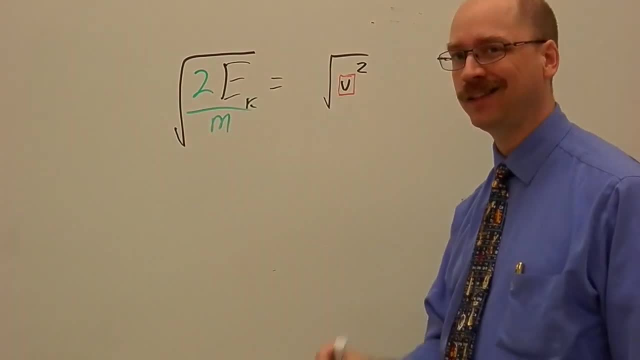 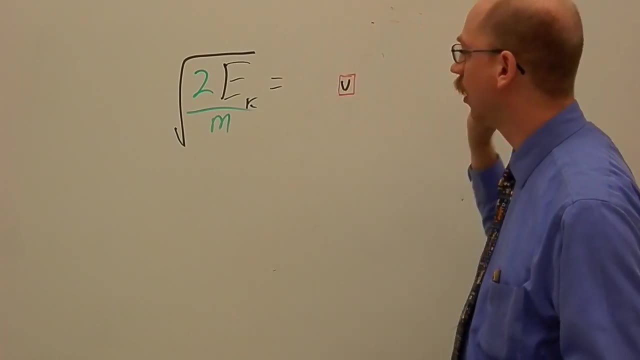 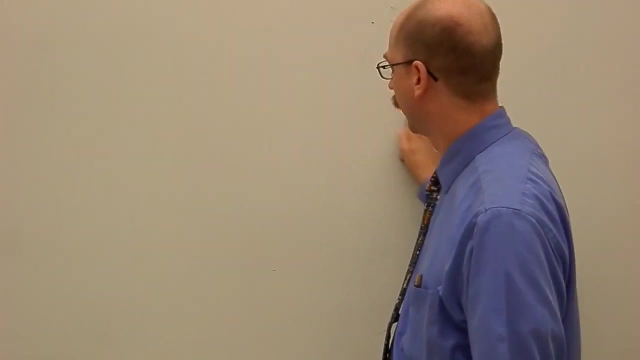 and all the way across, Because you have to show that that entire thing is being square rooted, Otherwise it's not correct. Over on this side, square root cancels the square and I'm left with V. Okay, Then there's some that look a little bit weird. 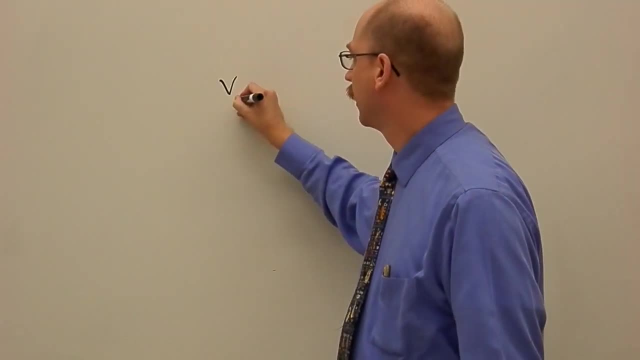 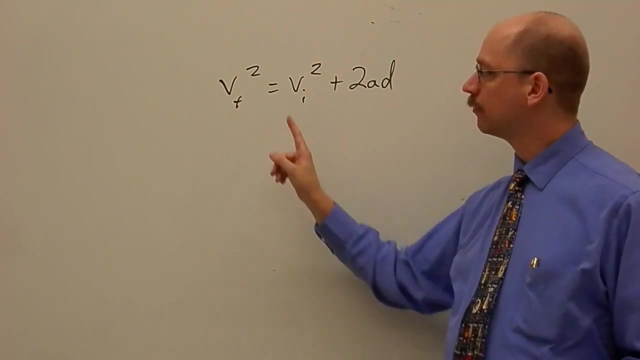 maybe because they've got some addition going on in them. This is a formula that we'll be doing in about one week. Okay, Okay, Okay, Okay. And this formula looks weird because from the very start they put down the unknown variable on the left hand side as vf squared. 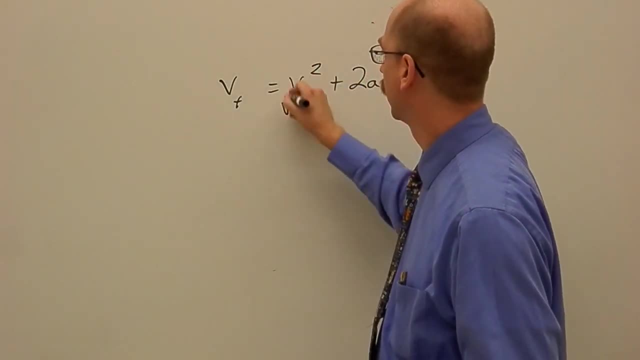 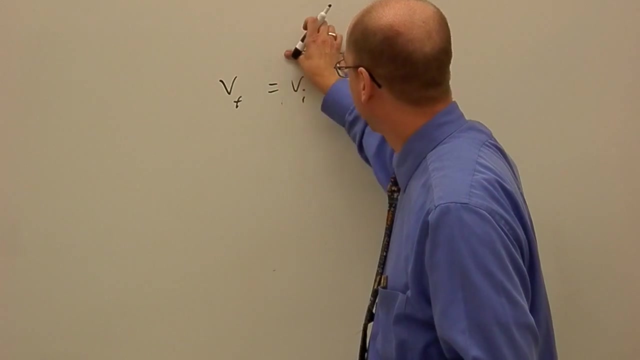 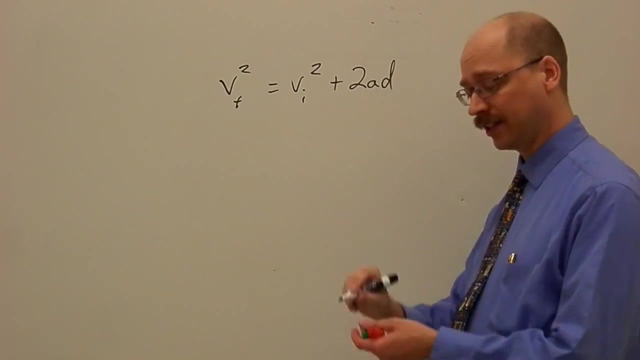 So if I was going for vf on its own, that's all I'm going to do, just square root everything, and I'm done. That would be solving for vf. If I needed to solve, though, for something like, let's say, a the acceleration things. 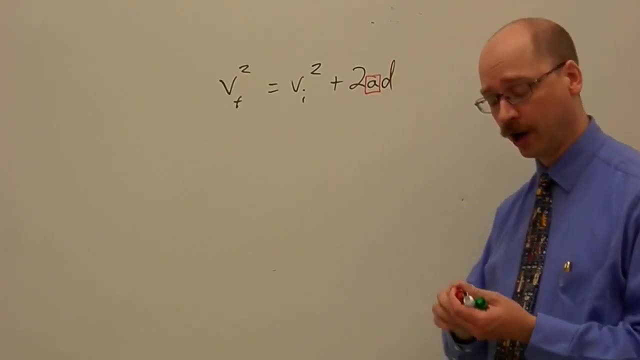 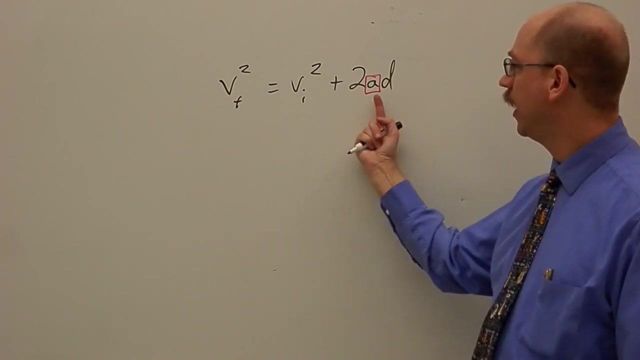 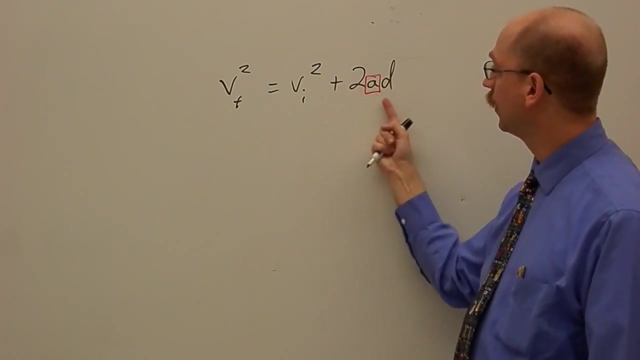 are going to look a little bit different Now. remember I told you earlier: try to do bed mass backwards. So I'm going to try to start with the addition and subtraction. Yeah, a is over here with 2 times d, but I'm looking at how, right now, the term that a is. 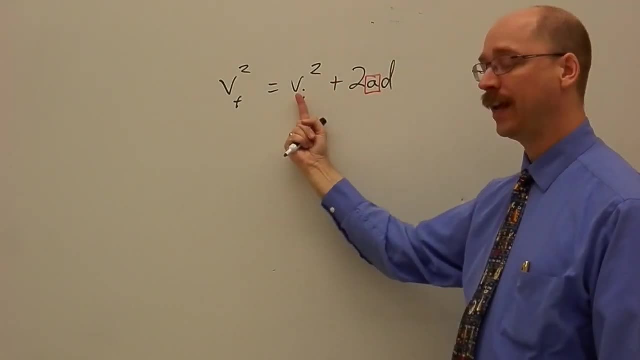 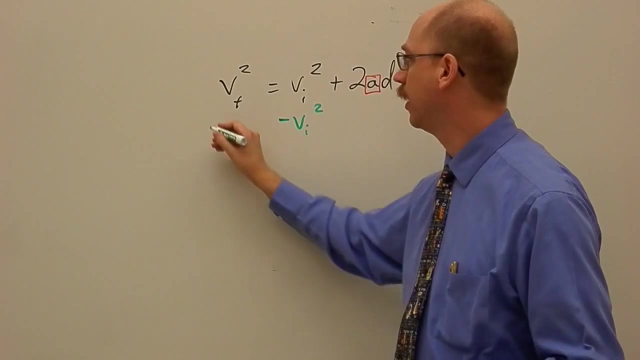 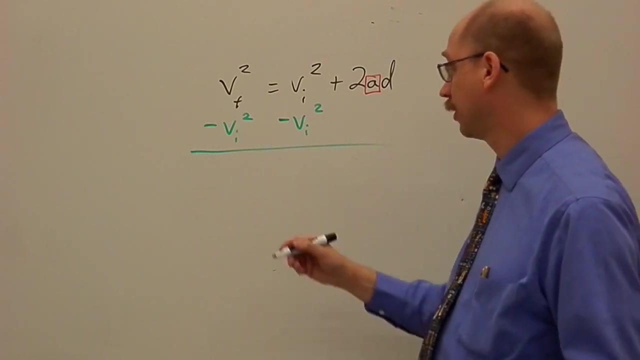 in. has vi squared being added to it. We take care of that first. We go ahead and we subtract vi squared and we subtract it from both sides. Quite often I've seen people do this. They go right out this way when they're doing math problems. same sort of thing for us here. 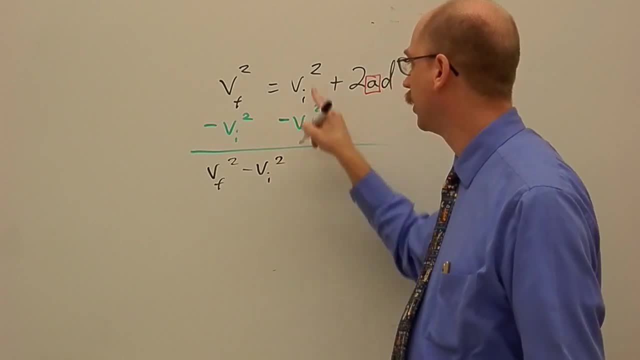 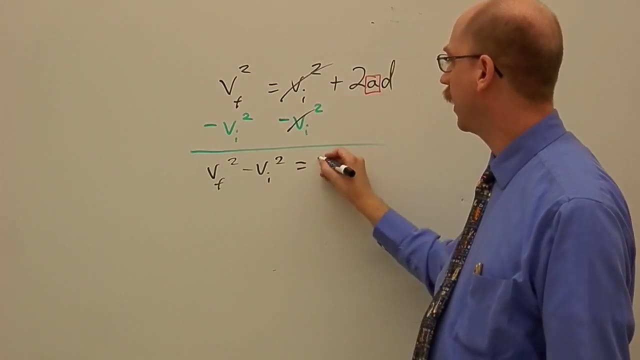 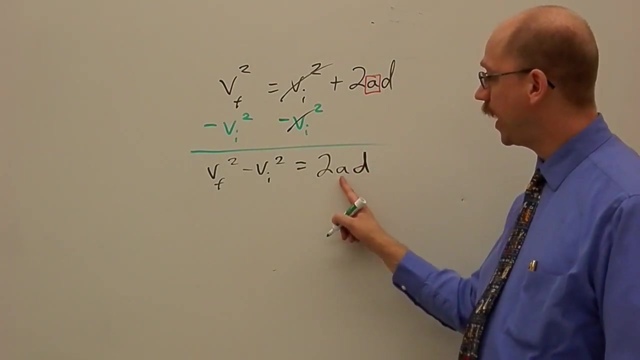 So we've got vf squared minus vi squared, because on this side it's vf squared minus vi squared. This part just cancels. So on the right hand side, all I'm left with is 2ad. Now remember, I'm trying to solve for a, and right now a is being multiplied by 2 and d. 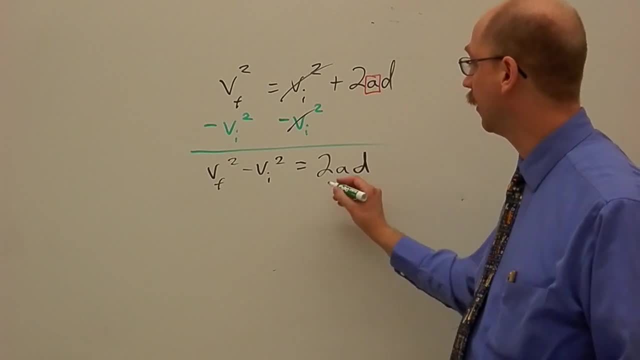 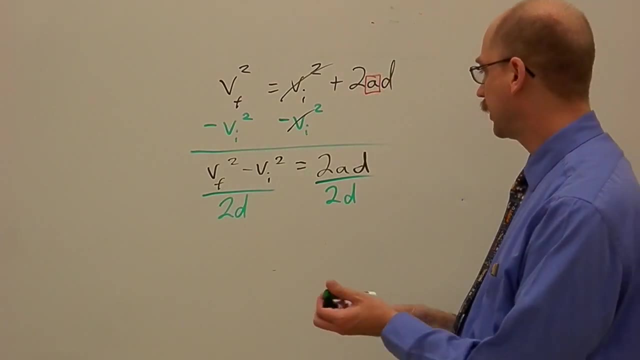 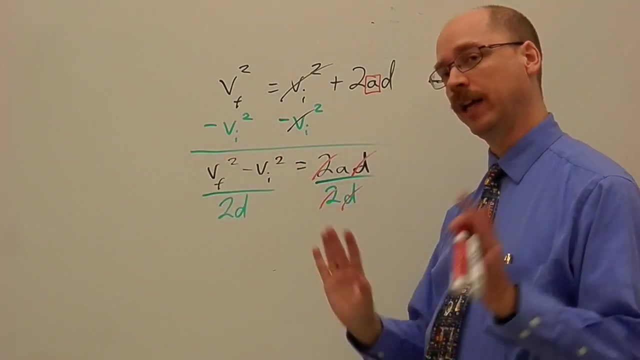 So I might as well take care of it all in one shot. There's no worries there. So divide by 2d, divide by 2d On this side. 2 and 2 cancel, d and d cancel, and nothing's cancelling over here. 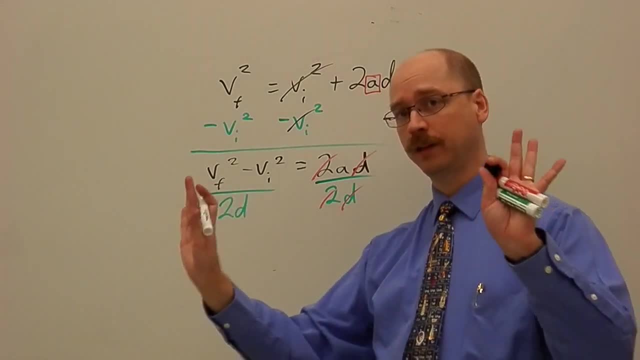 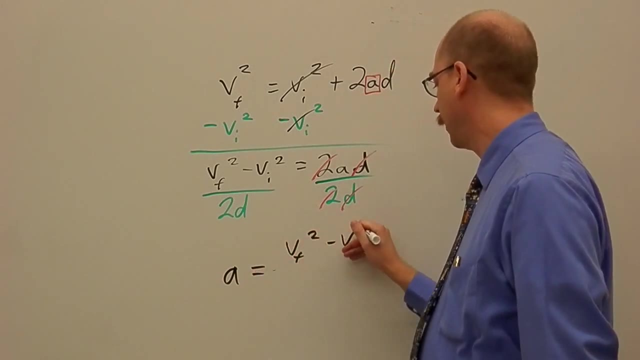 That stuff's just sitting there. I'm going to be left with a new formula and if I flip it around to get my unknown on the left side it's going to say vf squared minus vi squared over 2d. Looks like a big hunk of stuff, I know. 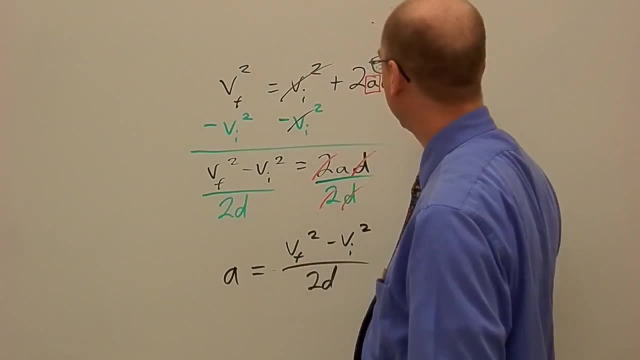 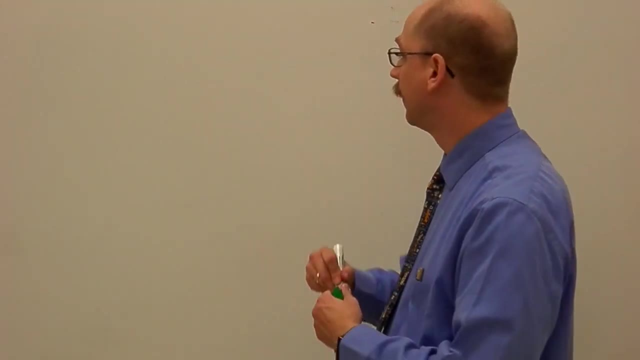 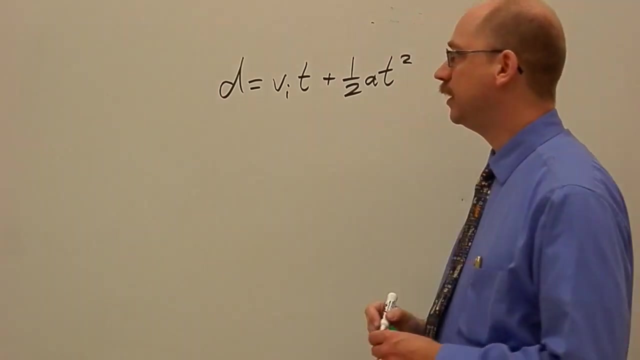 One last one that I'm going to get you to think about a little bit is one of the granddaddies of chapter one. It's one of the most important formulas that we've got: d equals bit plus 1 half at squared. 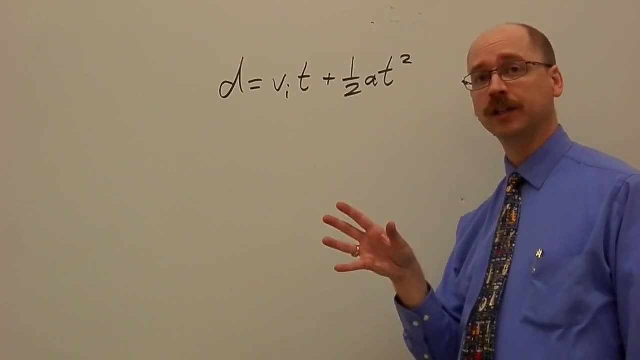 It is a monster and it means that you'd have to move around a lot of stuff. but I can do it, if I do it in little pieces. What I want you to try to do is: maybe you can do it in a little bit. 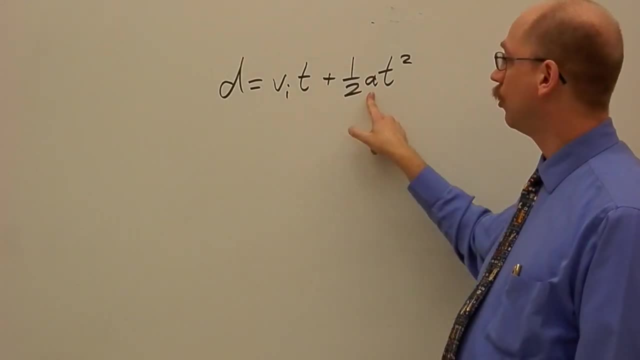 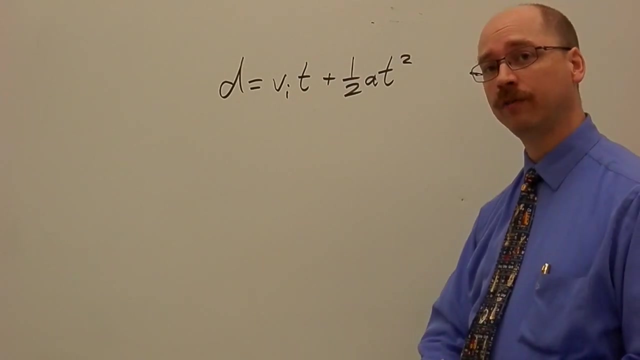 You can do it in a little bit. Maybe solve this for vi, Solve it for a, See what happens. But then- the weirdest thing in the bunch- Take a look at whether or not you can solve it for t. Some of you that might have done a little bit more math might know that that would involve. 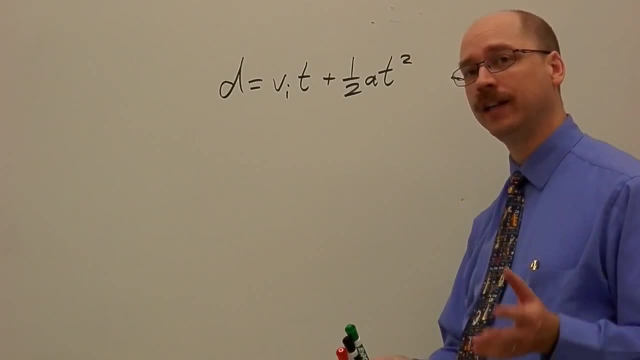 something called a quadratic, And what I can tell you is that in physics 20, we will not ask you to do questions with a quadratic, so you don't have to worry about that. Instead, we're always going to rig this formula so that, if you need to solve for t, you can.